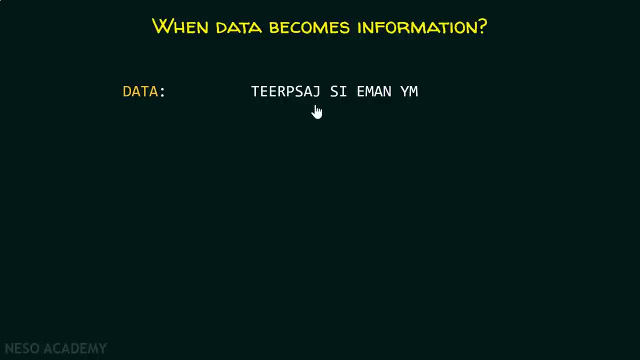 like this, or collection of symbols like this, then this is just a data. because it is just a collection of characters, I won't be able to understand it properly, right? Would you be able to tell me what exactly I have written over here? No, right? 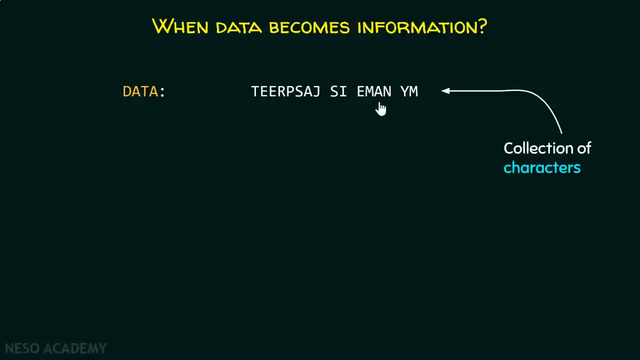 But when I process this data and let's say, I reverse, this whole string means the last character becomes the first character, second last character becomes the second character, and so on. Then it becomes an information, because now I can read this and I can understand what is written Here. I have written: 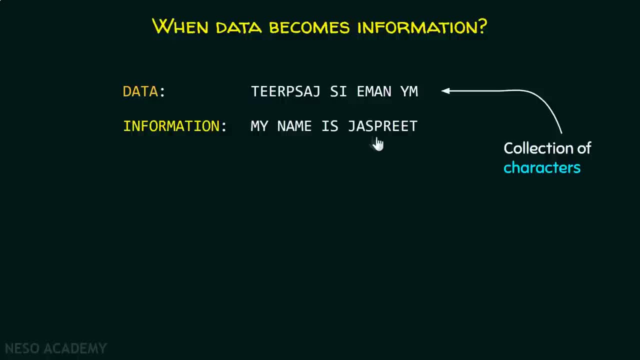 the name is just breathe, So it is quite understandable. So I can say that now here data becomes information because I can extract some meaning from it. So if data is arranged in a systematic way, then it gets a structure and become meaningful. 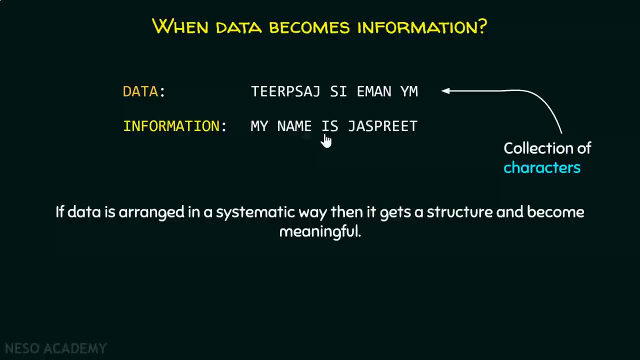 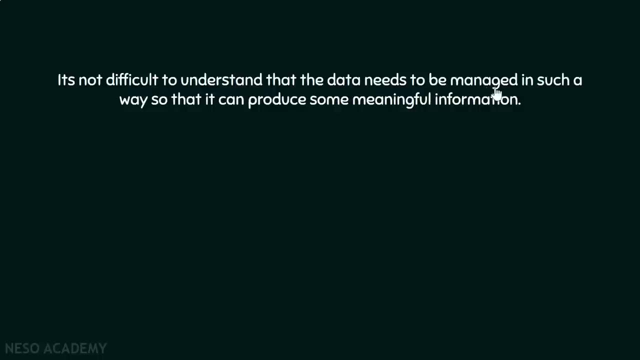 Here I have arranged the data in such a way that it becomes meaningful for me. Therefore, I can say that this meaningful or processed data is called information. Now, it is not difficult for us to understand that the data needs to be managed in such a way so that it can. 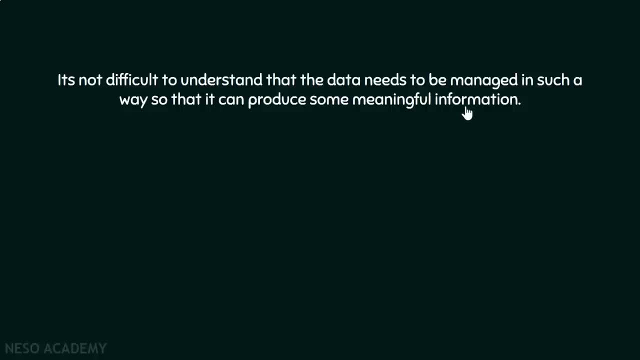 produce some meaningful information. We need to arrange our data. we need to manage our data in such a way so that we can produce some meaningful information To provide an appropriate way to structure the data. we need to know about data structures. That is why it is so useful to understand. 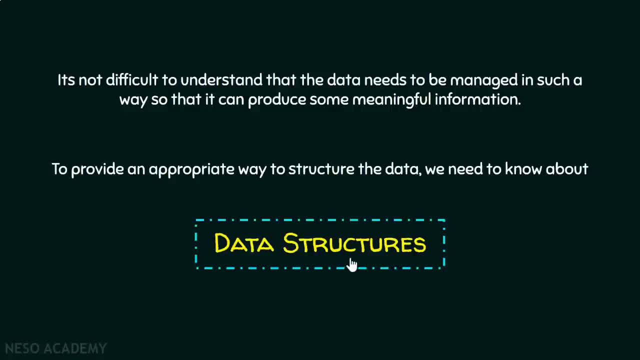 data structures. Data structure gives us the way to structure the data, to appropriately manage the data so that we can get some meaningful information from it. and not only that, we can use it whenever required in an efficient way. This is the reason why companies are preferring 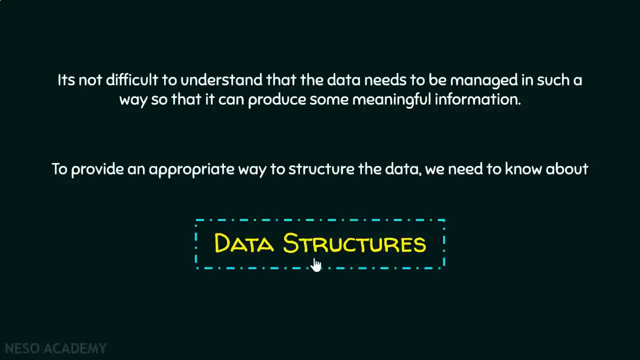 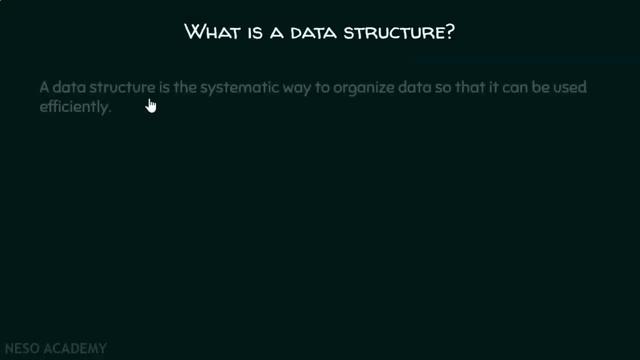 this subject over other subjects, because this is very important subject Right Now. let's understand what is a data structure. A data structure is the systematic way to organize data so that it can be used efficiently, So organizing the data in such a way so that we can use it. 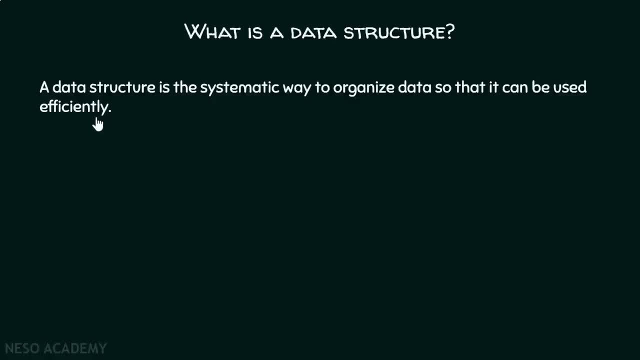 efficiently is what data structure is all about. We are arranging the data, we are organizing the data, we are managing the data in such a way so that we can use it efficiently. When I say efficiency, I mean in terms of time as well as space. Let's see one. 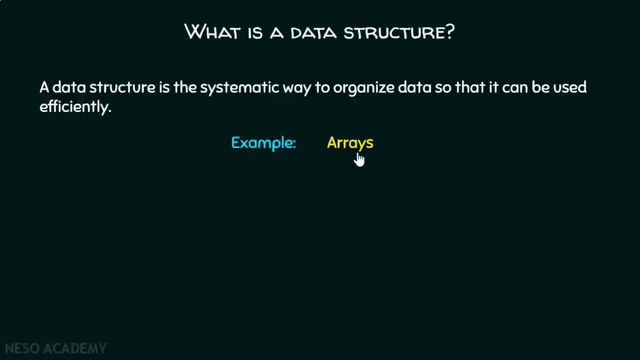 example of a classical data structure: Arrays. We have used it many number of times. We can think of it as a sequence or collection of some symbols, characters, integers, floats or something like that. Right, You can think of array as a data structure. 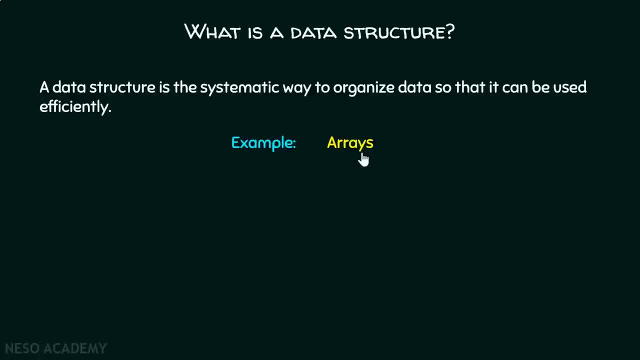 because it is helping us in managing the data in an appropriate way, actually in a sequential manner. Now here is an example why this data structure is so useful. Instead of creating multiple variables of same type, why not create an array to store all the values? Let's say: 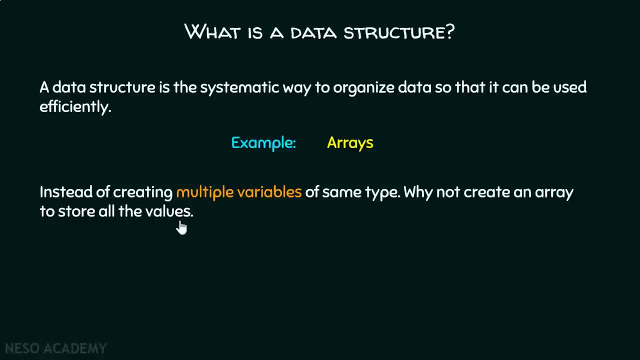 I need hundred integers. Why do I require to create hundred variables for hundred integers when I can create a single array and store all the integers in them? Isn't that so? That is why arrays are so useful. Or you can think of one example like: 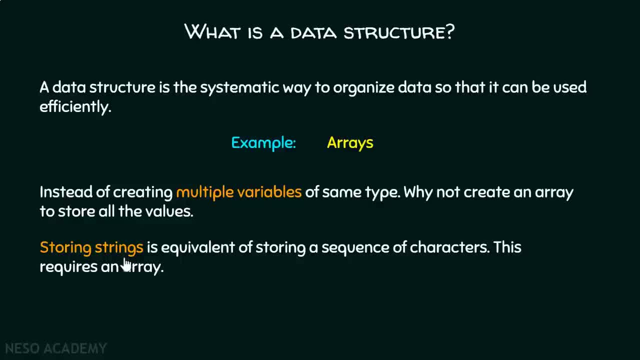 storing strings. You know that strings are nothing but sequence of characters. Right, Let's say a string consists of hundred such characters. Now are you going to create hundred variables for that? No, You can create one array which can store that whole string, and we would be able. 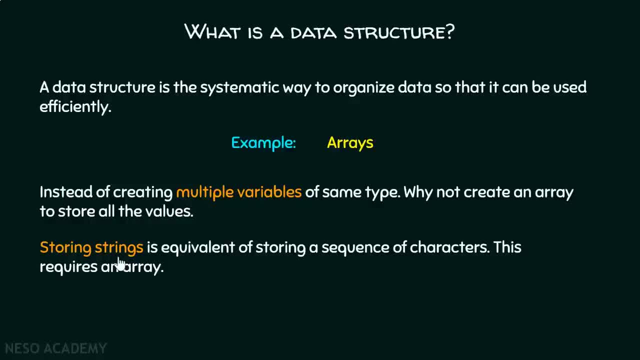 to access it very easily, Isn't that so? So this requires array, and that is why we need arrays, because it helps us in managing our data in an appropriate way. That is why it is a very useful data structure for us. Now, 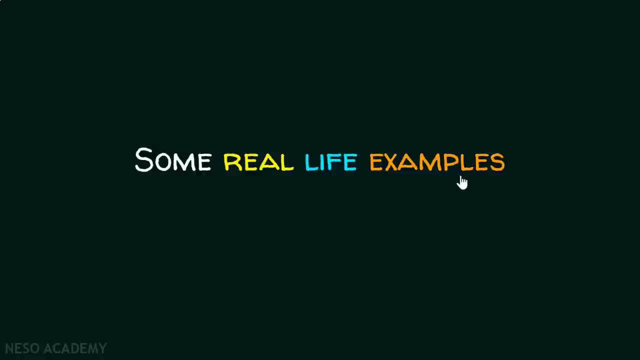 let's discuss some real life examples of data structures to help understand why do we need data structures. Here is an example. Did you know that stack data structure is used in implementing redo and undo feature? You know this is the famous feature which we are using many number of times. 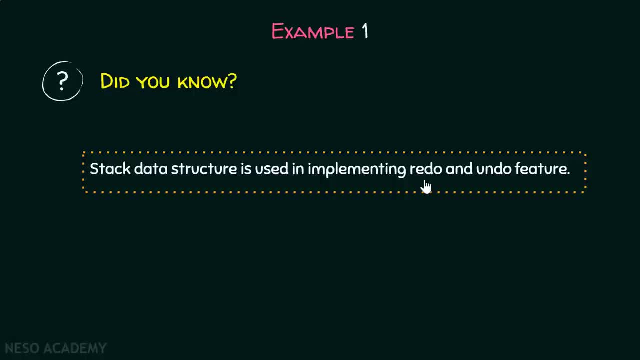 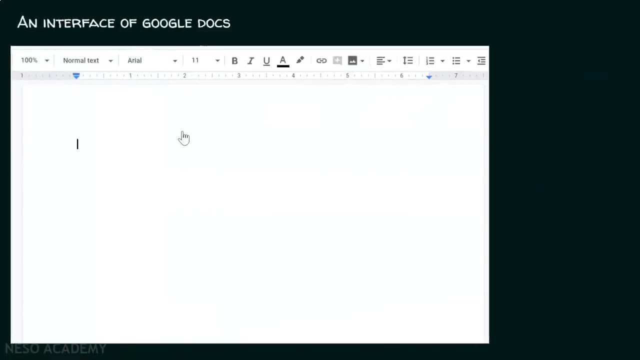 in our applications right. One such application is Google Docs or PowerPoint or Microsoft Word. Redo and undo feature is very famous, But did you know that stack data structure is used in implementing this feature? Let's see how. Here I have taken an interface. 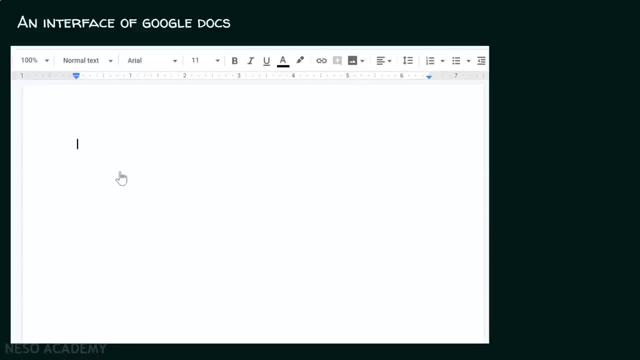 of Google Docs. Here I am going to write something. Let's say I have written. the primary goal of the academy is to give quality education. I want to write education here, but I forgot to mention here U, So instead I have written education, something like that: 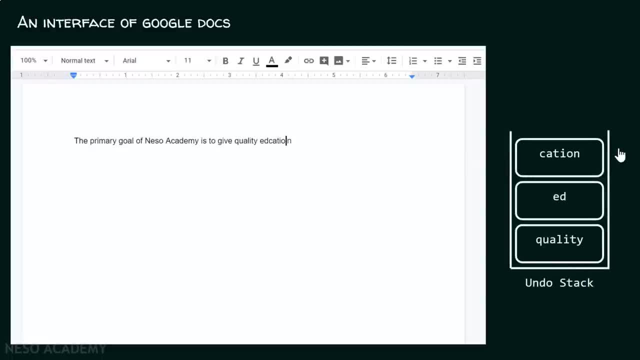 Let me tell you that here a stack is maintained where each and every information that I have entered gets stored, Like in this case: quality is stored, ed is stored separately, cation is stored separately. So this is our undo stack. We know that in stack. 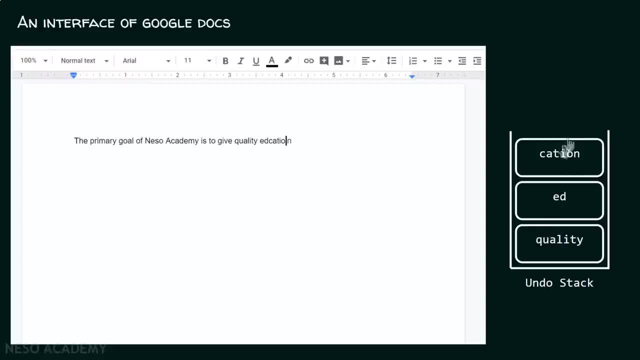 the data is placed from top and whenever we want to get the data, we can get it from the top. Only the top element we can access right Now. when I press control z then I know it means undo, right, So what it does. 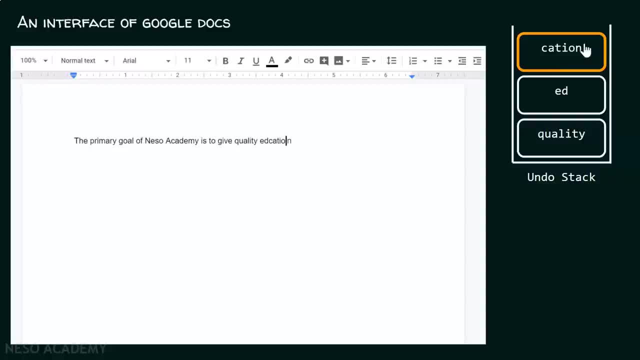 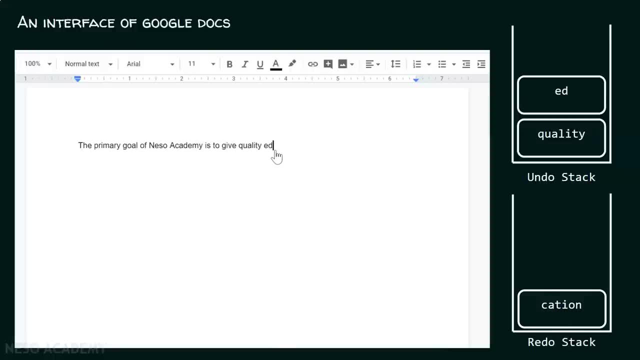 is it selects the top element and it pops that element out of the stack and placed it in the redo stack. That is why we can see here that cation get removed when I press control z. Control z means undo the operation which I have performed. 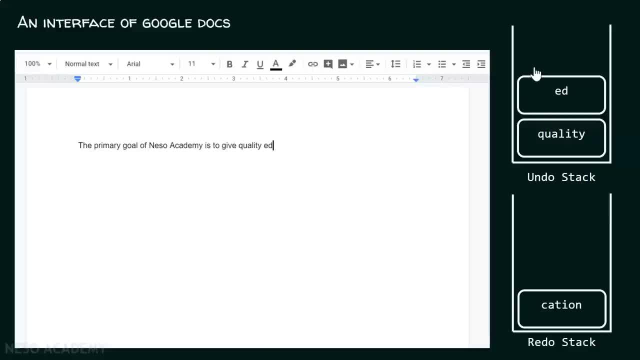 Here, in this case, I have entered cation. I just can remove that out of the stack and then after that that particular element will get placed within this redo stack. Why it is placed in this another stack? Because when I press control y, that is redo. 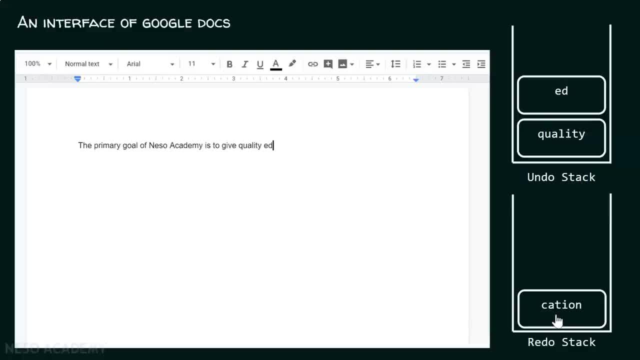 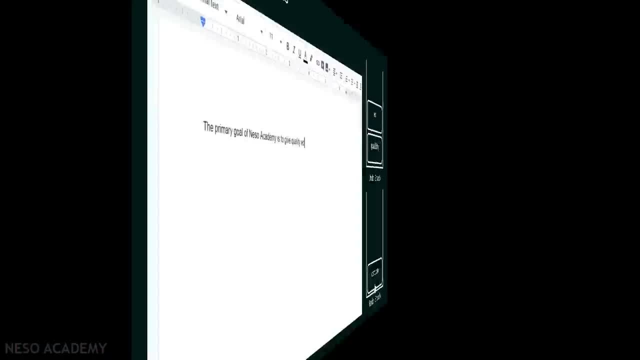 then we can get that again. That is this cation. I would be able to get that again over here. Maybe I want to redo my operation. That is why redo stack is also required. Now I can continue writing. I have written the primary goal of. 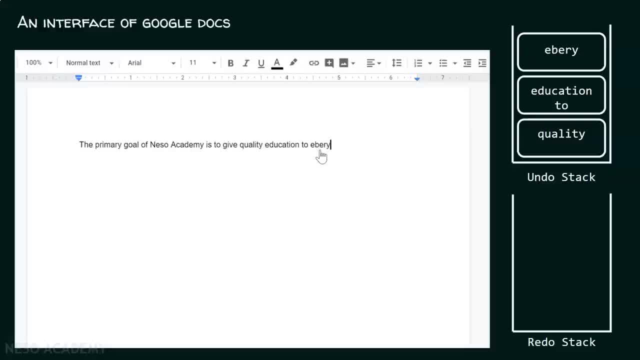 Neso Academy is to give quality education toactually I want to write everyone, but accidentally I have written every instead of every. I press control z. this element gets selected and you know it will get popped out of the stack and will get placed within this redo stack And you can. 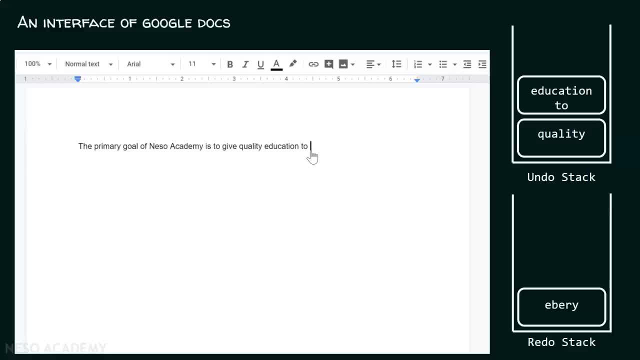 see here, the operation is undone Right Now. let's say I want to redo the operation. When I click on control y, then this particular element gets selected and it will get popped out of the stack and will get pushed within this undo stack once again. 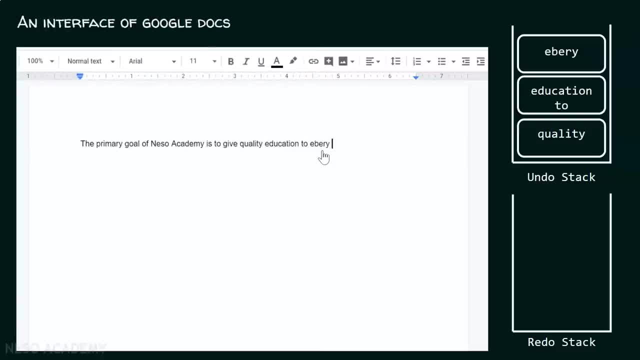 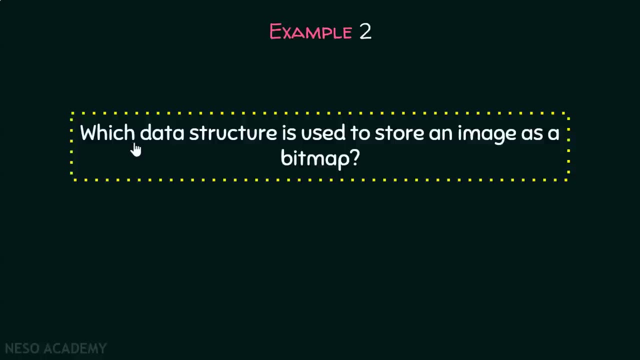 So here the operation is redone. This is how undo redo feature works, And this is one such application of data structure, And you can see here: stack is our data structure. Now let's see another example: Which data structure is used to store an image. 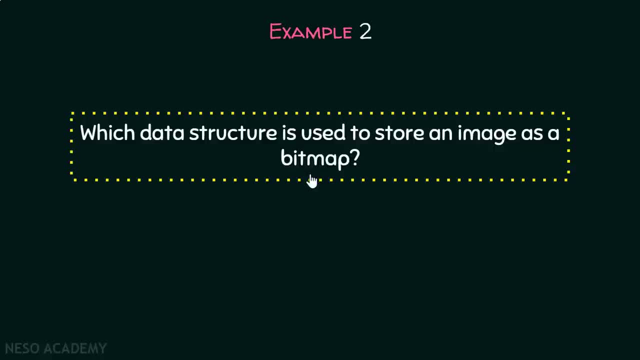 as a bitmap. Do you know which data structure is used to store an image as a bitmap? There are two types of images: bitmap images and vector images. Now, when I talk about a bitmap image, do you know which data structure is used? 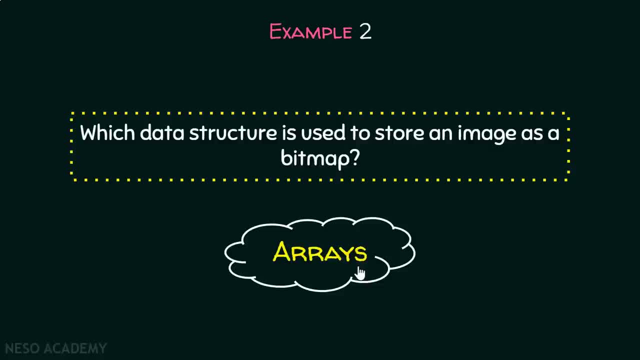 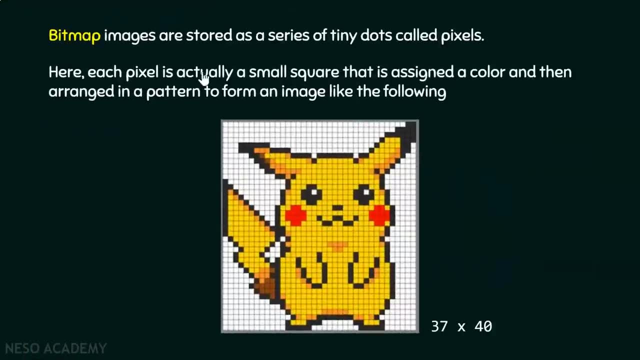 to store that image. Guess what It is? an array. Array is so useful that it is used in storing an image as well. Let's see how Bitmap images are stored as a series of tiny dots called pixels, Right? So here you can see in this image. 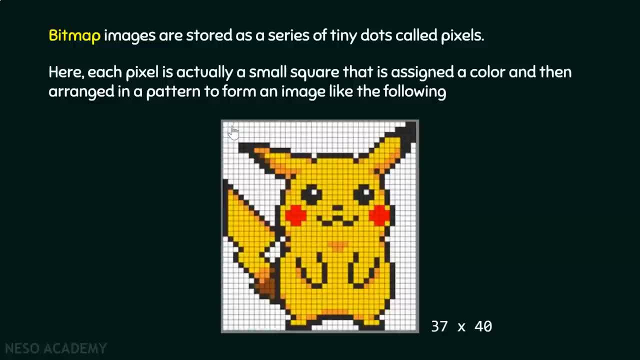 that these tiny dots or squares are called pixels. Here, each pixel is actually a small square that is assigned a color and then arranged in a pattern to form an image like the following. So you can think of a two dimensional array like this Here, in this example. 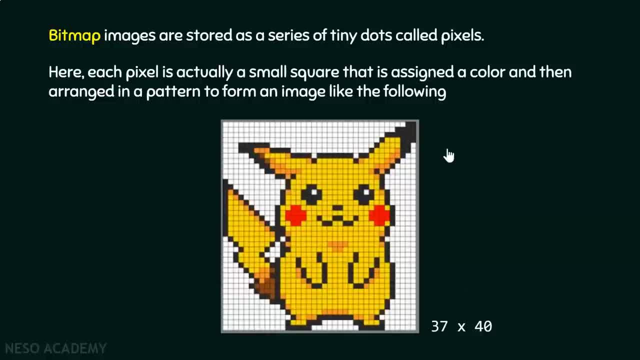 it is thirty seven cross forty. Now, within that two dimensional array, you are storing pixel information, That is, each pixel color you are storing and then, after that, you are arranging it in a systematic way and finally, we get this as a result: That is an image of a Pikachu, Right. 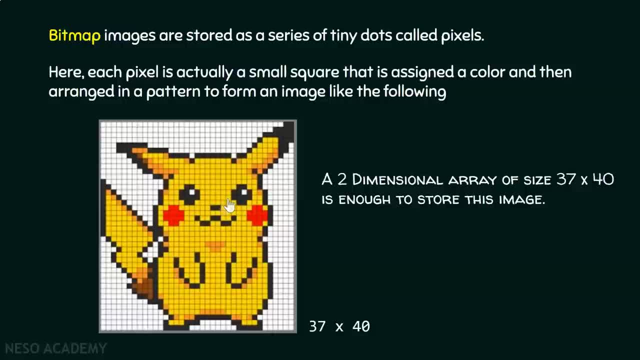 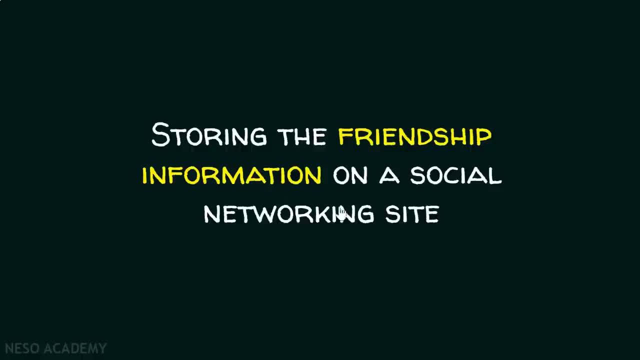 So a two dimensional array of size thirty seven cross forty is enough to store this image, Isn't that? so Now let's see our example number three: Storing the friendship information on a social networking site. Do you know how Facebook is storing the information of friends? 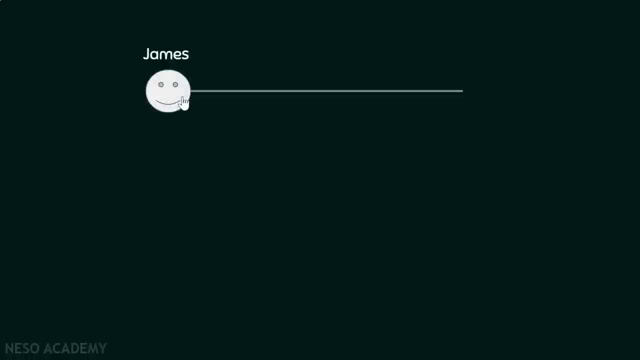 Let's see an example here. Let's say, James is a friend of Mark. Not only that, James is friend with Leah as well. So here we are: maintaining the connections between them. This particular edge is representing the relationship between James and Mark. 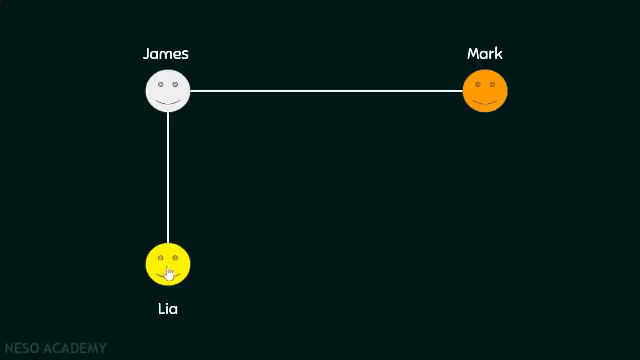 Okay, Similarly, James is friend with Leah, and it is represented by this edge. Not only that, Lucy is friend with both Mark as well as Leah. So here I am maintaining the connections like this, But it should be noted that James and Lucy are not friends.